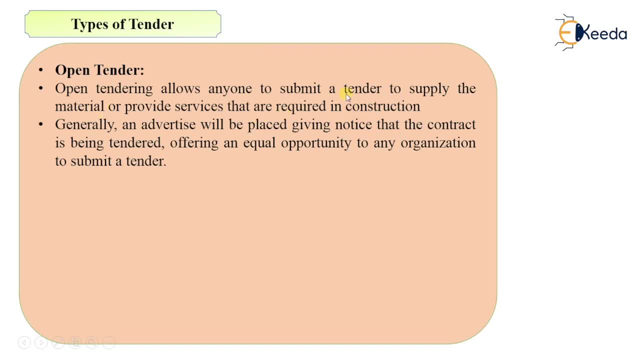 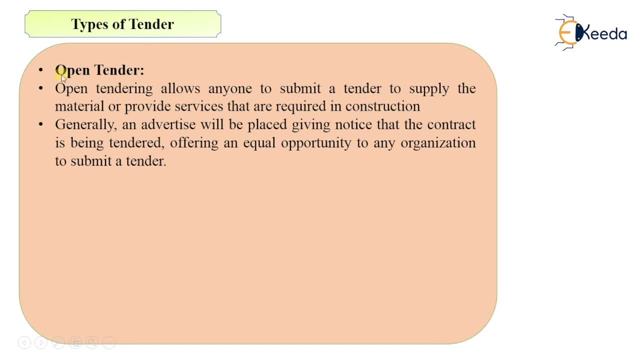 equipments will be required for that particular work. so it is not not like that. it is open to all and generally an advertisement will be placed giving the notice that contractor is being tendered. they will be giving an advertisement in the newspaper that contract is being tendered. 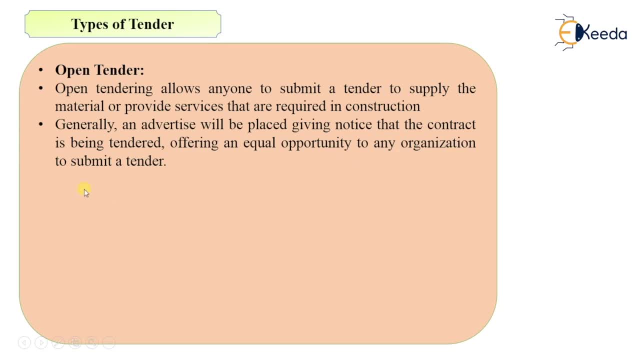 offering an equal opportunity to any organization to submit a tender. any organization can apply for that particular tender and open and open tendering is performed in both the private and government sector. we can use it, this type of tendering. it is generally used for both cases in private sector. 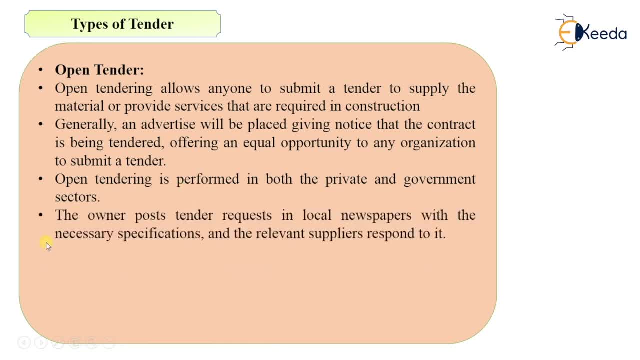 as well as in government sector. we can use this type of tender and the owner post tender request in local newspaper with the necessary specifications and the relevant suppliers respond to it what he will do. the owner who wants to execute his work or who wants, who wants material for the construction. 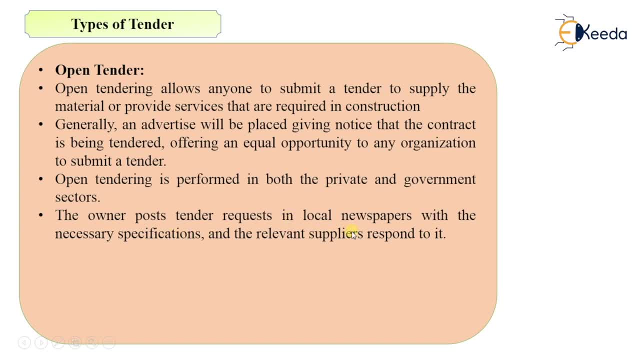 of particular work. so he will request in local newspaper with necessary specifications, that this, this, this is my requirement. i want to complete my project in this this days. so if anyone is interested, they can code their rates so they can't apply for that particular tender and they will times that you will find a. 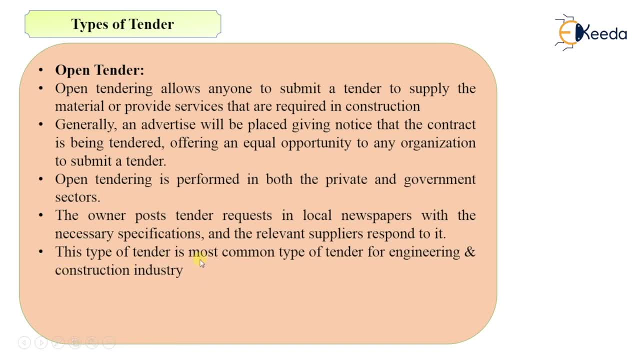 man who has been producing or producing tender with this result and that tender and we take reference them out to that particular it. so if you are in the Ship, maybe when the there will be a tender dawn or bigger tender coming next year, etc. and little depends on that is. 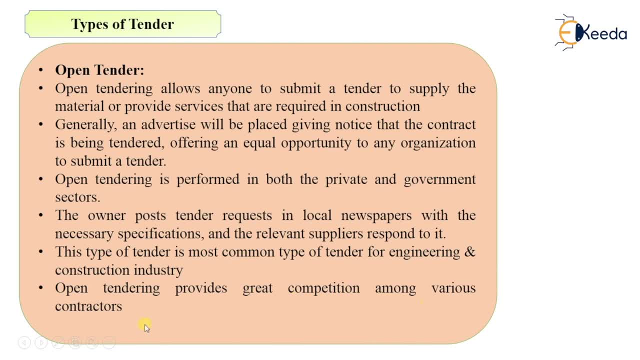 what you are showing us now. more related to that, then take a look in the description. what it is. property for me. the name because it is open to all. anyone can submit this tender, so it is very competitive now. 254 gray 385. whatever is given to us, it is to make sure. 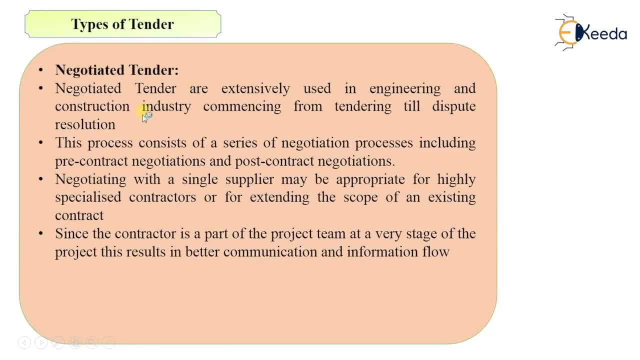 Now the next one is negotiated tender: see negotiated tender. negotiated tender are extensively used in engineering and construction industry, commencing from tendering till dispute resolution. this type of tender is very helpful and it is extensively used, widely used in construction industry, from tendering process till the dispute resolution. this can be used and this process 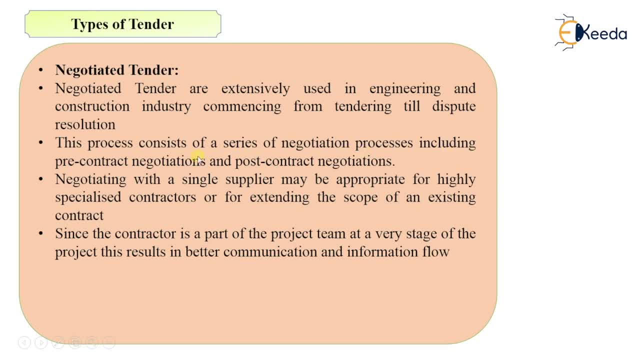 consist of series of negotiation processes, including pre-contract negotiation, post-contract negotiation, because, as the name says, it is negotiated tender. So there will be negotiation process before the contract, that is pre-contract negotiation. will be there post-contract after the contract has been signed, that is post-contract negotiation. 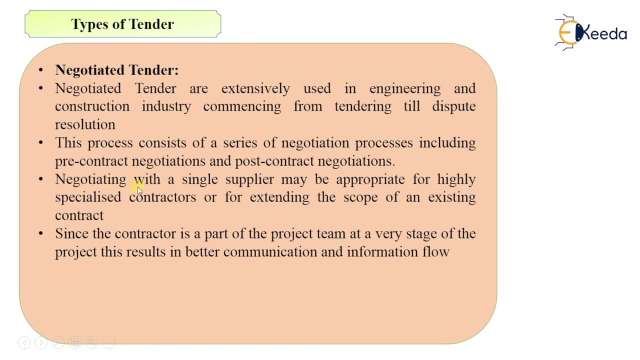 So, as the name says, negotiation will be there. so negotiating with a single supplier may be appropriate for highly specialized contractors or for extending the scope of an existing contract. see negotiate. if you want to negotiate with someone for single supplier, it is a single supplier. it. 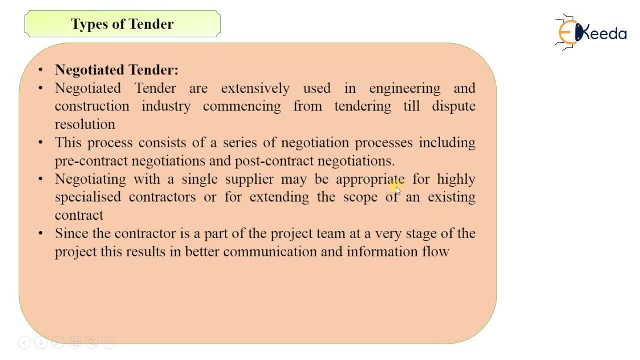 will be very good. it will be very appropriate. for example, there is some highly specialized contractor. he can fulfill your demand. he can execute the work for you- construction work- for you- or he can supply the material in a very good rate. so you can negotiate with him by the. 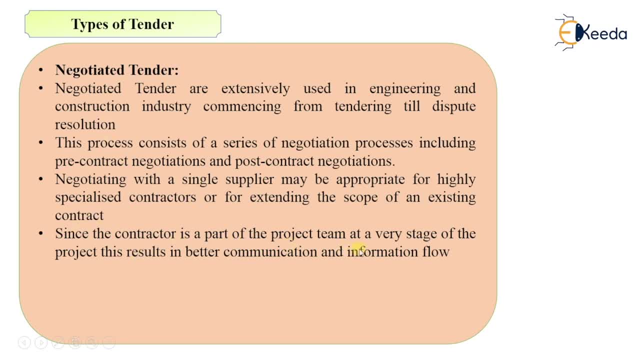 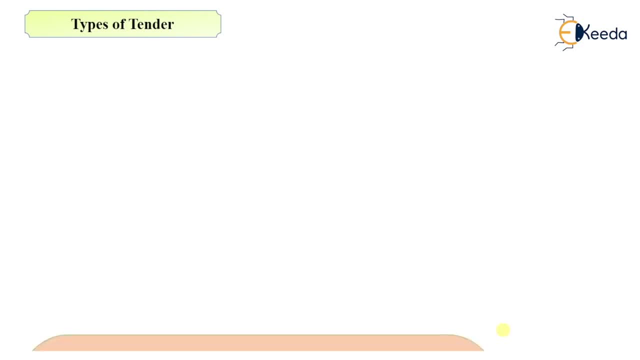 negotiated contract, since the contractor is a part of the project team at a very stage of the project. this results in better communication and information flow. this type of tender. now the next type of tender is selective tender. so what is selective tender? see, selective tendering only allows suppliers to submit. 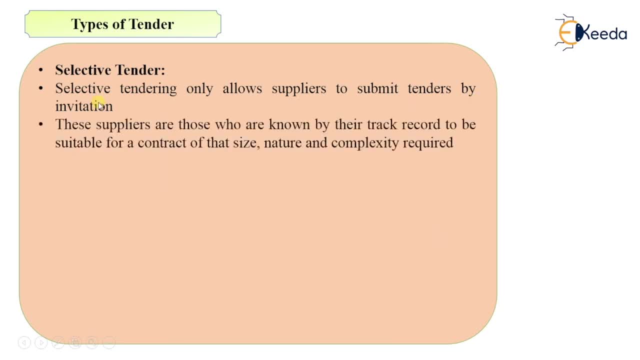 tenders by invitation. this type of tendering will allow the suppliers to submit the tenders only by the invitation they will be invited. this suppliers are those who are known by their track record to be suitable for the contract of that particular size, particular nature and complexity. 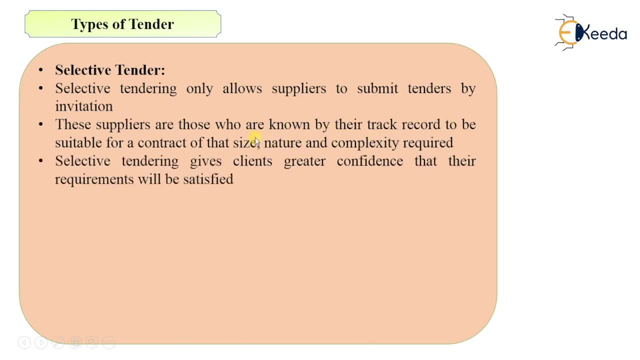 required means. there is some work which cannot be offered to a common tender, common contractor. so this type of tender will allow the suppliers to submit the tenders only by the invitation. it may require some special skill or some past experiences or the contract will be very big. that. 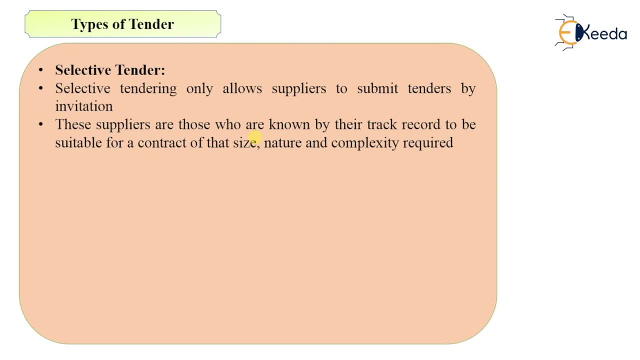 small contractors cannot complete it, cannot execute it, or you cannot give it to the new contractors because of its nature, because of its complexity. so what you will do, you will invite selected contractors only for completion or for execution of that particular work or for supply of materials, whatever it is so that contract, that tender is called as selective tender and selective tendering. 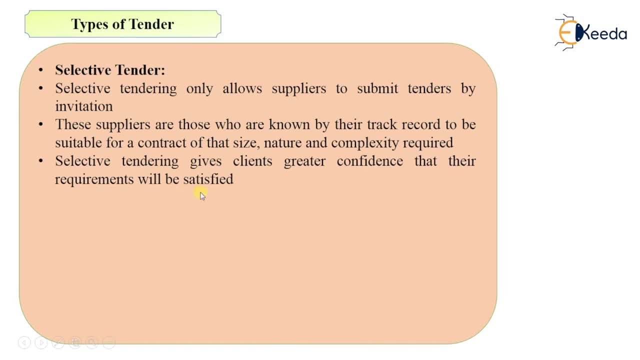 gives clients greater confidence that their requirement will be satisfied, because they have in their hand now that whom to select, who they can select. for example, a particular contractor can fulfill the requirement or not, that they will know, so they can send the requirement. or they can select that particular contractor. so they have the right to select that particular contractor. so they can. 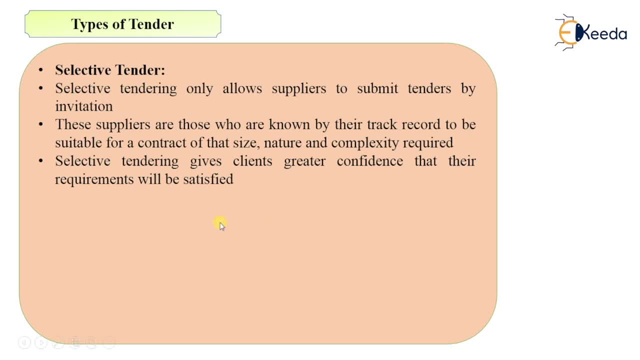 have that feasibility, so they will have confidence that the requirement will be satisfied and fulfilled. and it may be particularly approximate for specialist or complex contractors where there are only few suitable forms. it may be very particularly approximate because there are some specialist, there are some complex contractors. they are very few, okay. so, however, it can exclude smaller suppliers for those trying to 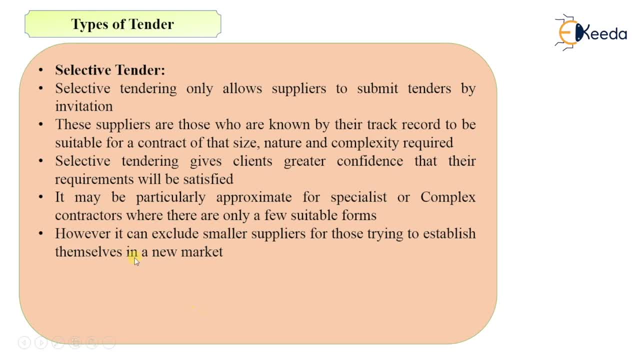 establish themselves in a very complex way. so it is a very specific requirement. so it is a very specific requirement in a new market. there is one disadvantage. you can say: those contractors which are new, they have talent, they can fulfill that requirement, they can execute that work, they can supply the material. 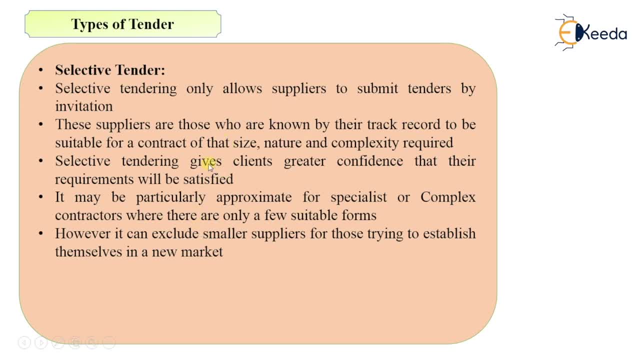 which that particular owner or client want. but as they are new, they will not be considered. so that is one disadvantage for selective tender. that is one disadvantage you can say, and selective tendering is an invitation to selected suppliers. only, as i told you it, they will be have invitation. 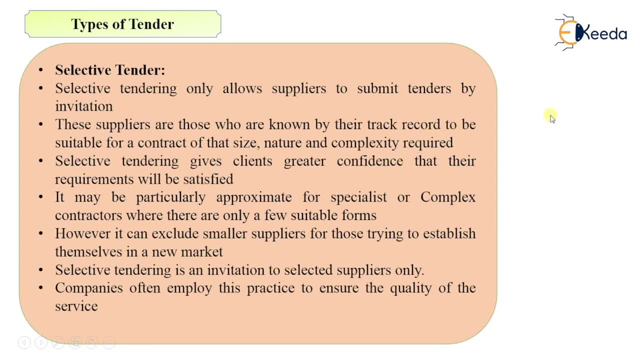 that this, this is work suitable for as per you. so you are invited to submit the tender for that particular work. companies often employ this practice to ensure the quality of service. those companies which you, which want quality work for particular work, they will employ this type of method. then the next method. 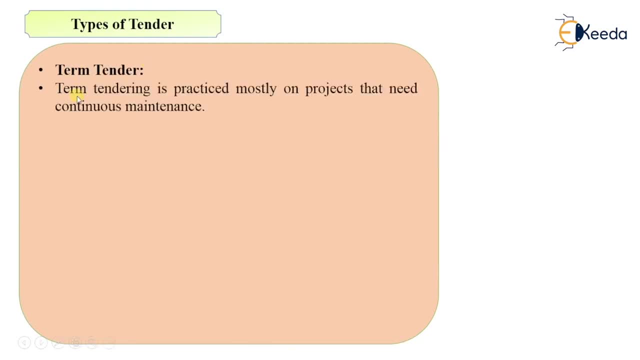 you or next type term: tender term tender is practiced mostly on projects that need continuous maintenance. for maintenance work, we will use tender which tender term tender. this often comes with definite time constraints. as the name says, it will have some term time limit, definite time constraints will be there and the project has to be completed within predefined schedule. because it is a 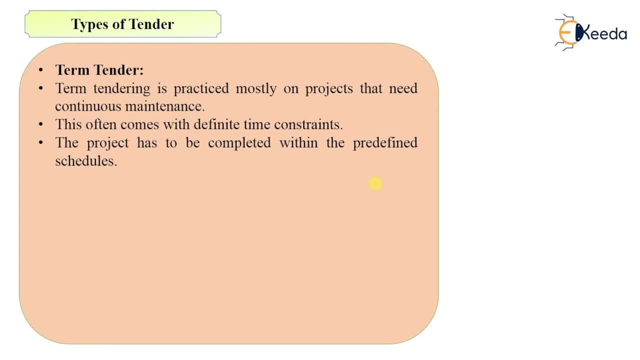 term tender. the project has to be completed within the predefined schedule and term. tendering usually refers to the process where governments and private firms invite bid for the large project that must be submitted within a definite deadline. there will be definite deadline in which government and private firms invite the bids for lar projects and 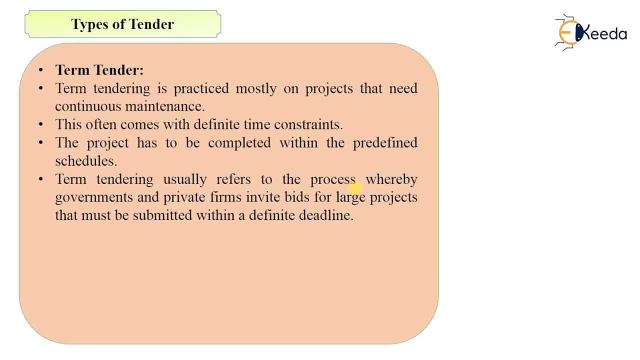 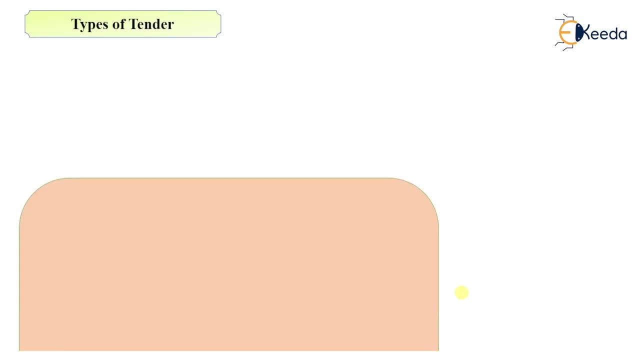 that must be completed and that must submitted within the definite deadline by the contractor. Now the last type of tender is limited tender. This type of tender see what it is. limited tender is addressed to a limited number of contractors and only those can code their rates. 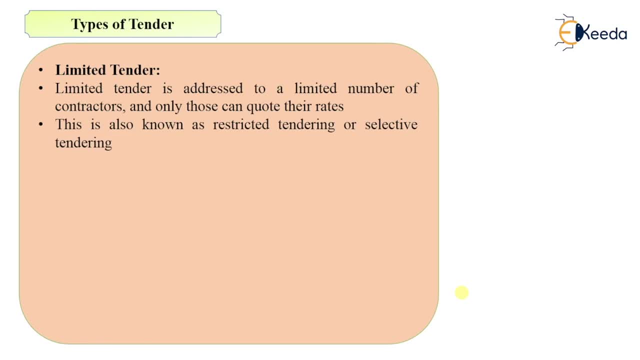 This type of tender will be limited to only limited number of contractors, limited number of people, and only they can code their rates, And this is also known as restricted tendering. as it is a limited tendering, So this is also known as restricted tendering or selective tendering. 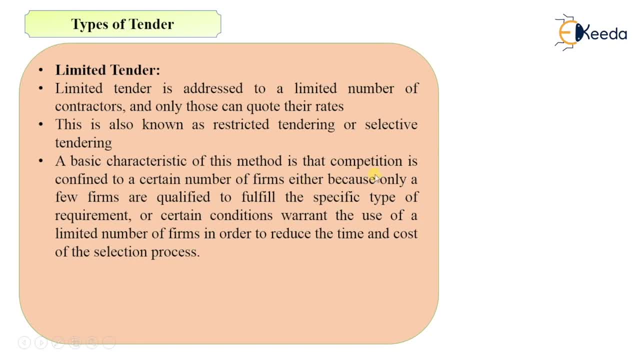 And see. the basic characteristic of this method is that competition is confined to a certain number of firms, either because only a few firms are qualified to fulfill the specific type of requirement, or certain conditions Warrant the use of a limited number of firms in order to reduce time and cost of selection.